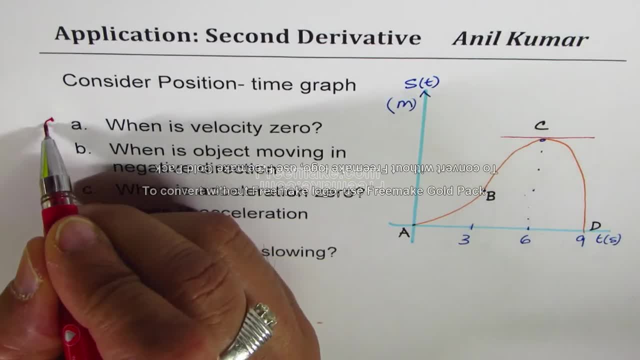 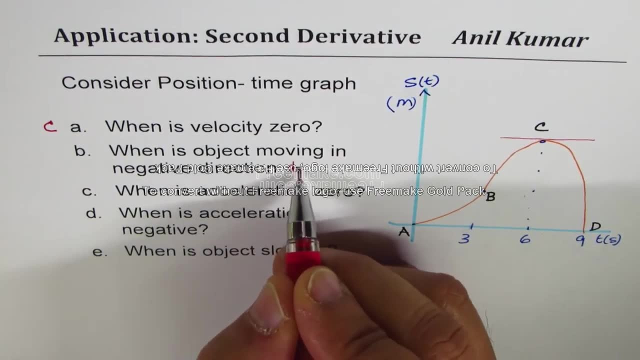 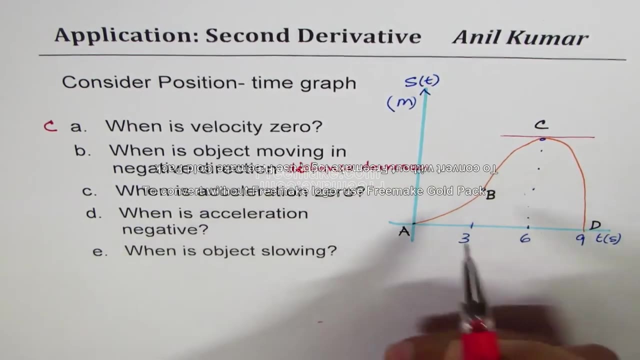 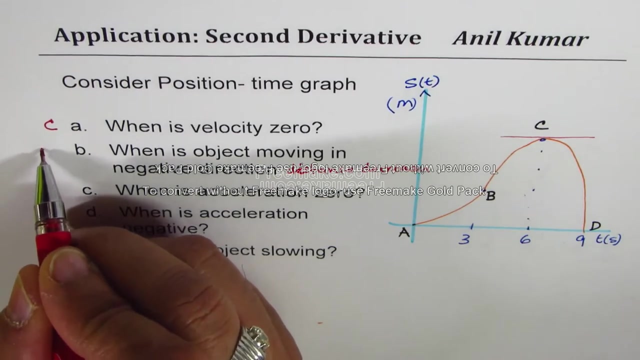 point is C, So let me write down the answers on the side. So it is at C. When is object moving in negative direction? Negative direction means distance, I mean decreases, right Decreases, So here it increases, but from C to D it is decreasing And therefore it is from C to D. 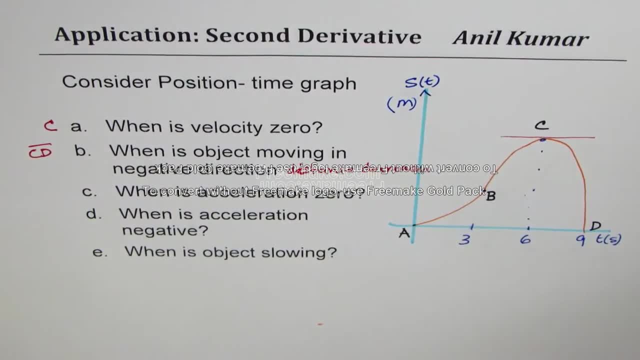 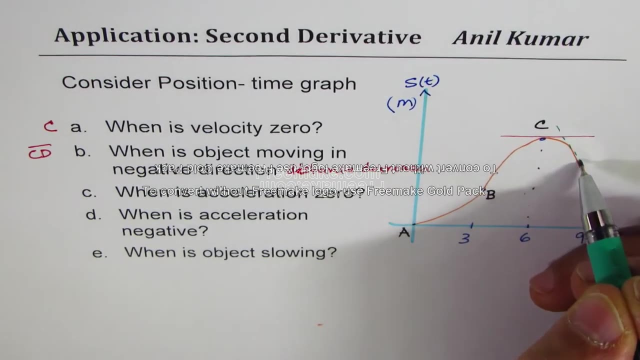 right. So that distance is decreasing, So the object is moving in negative direction. Also, whenever object moves in negative direction, velocity is negative. Is it okay? So if I draw a tangent line, the slope will be negative. So any tangent line during this. 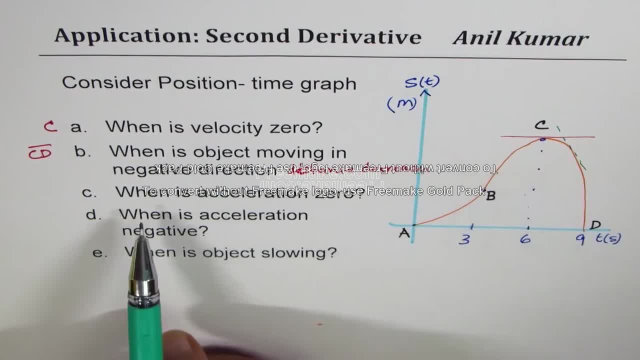 part will have negative slope When is acceleration zero. So either it could be a straight line here we have curved, So acceleration is zero at point of inflection. The only point of inflection here is point B, And so B is the point where acceleration is zero. 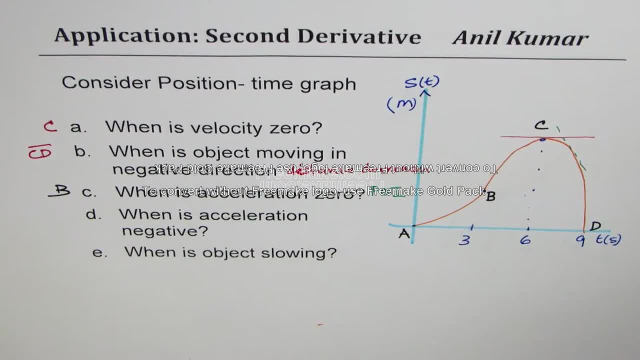 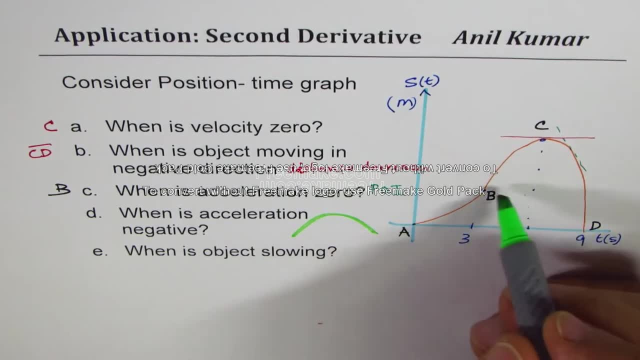 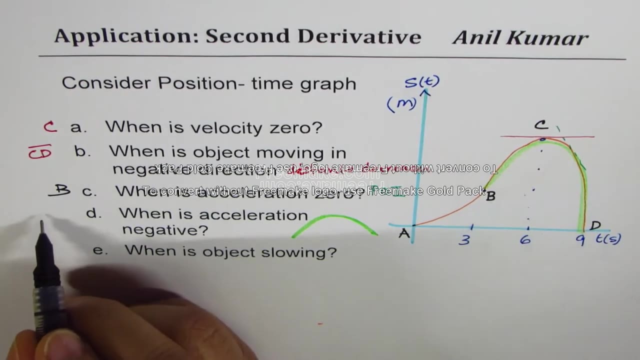 When is acceleration negative? Negative acceleration means we are looking for a curve which is concave down. So you can see: from B to D it is concave down, So we can say: from B to D, so B to C. right, So that curve. 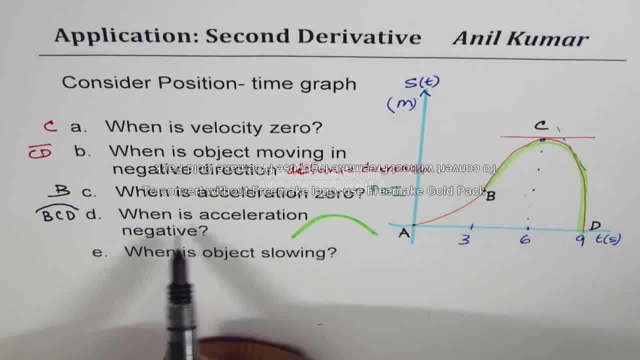 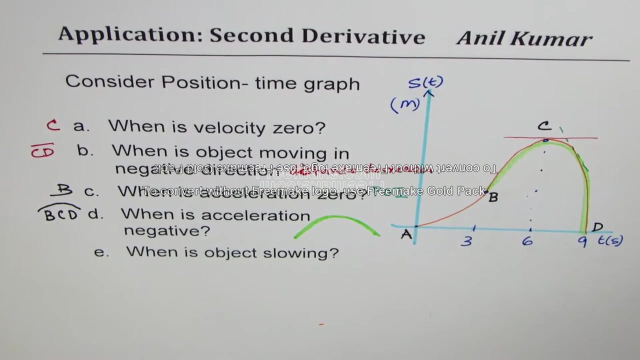 is the region or interval where acceleration is negative. The last question here is: when is object slowing down? So when is object slowing down? how do we get from the given figure? Now, object slows down when the velocity is zero to x-8.. So let's write down when object slows down. Object slows down when: 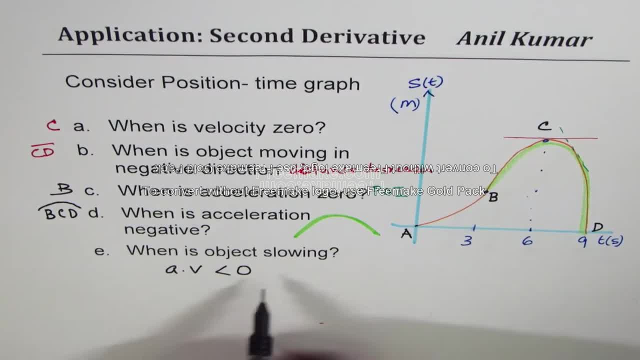 acceleration times. velocity is less than zero, So that means they have opposite signs. Is that okay? So that requires some analysis on this particular graph. Okay, let's do that. So this is a huge question. Okay, Let's try to understand. 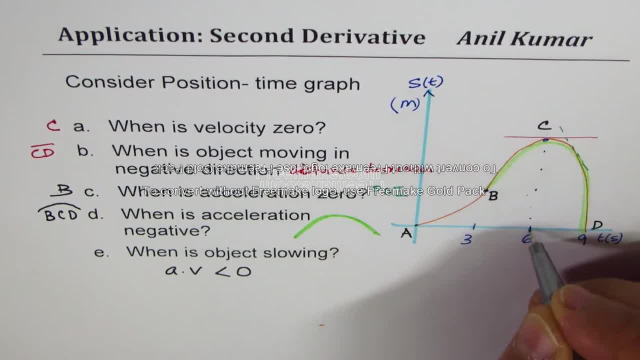 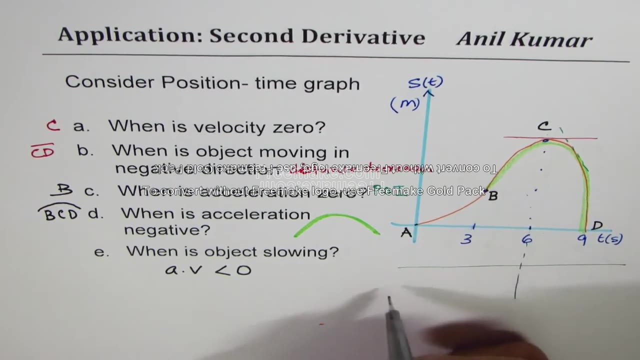 Okay, let's do that. So let's try to understand. Okay, let's try to understand. now, when does it slow down? okay, so we'll have to figure out. where is velocity positive? as you can see, velocity is positive, so let me make. I'm just thinking how to explain this. okay, so, okay, so what? 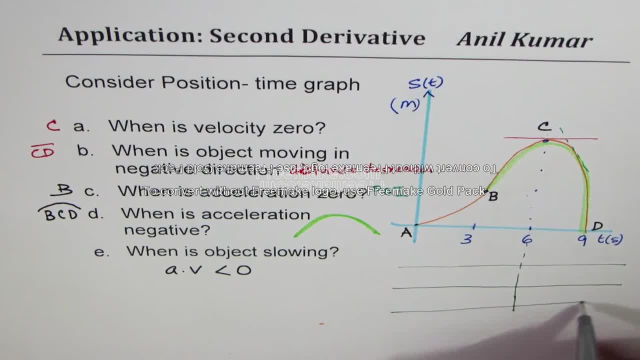 I will do here is: I will write down where velocity is positive and where acceleration is positive. right, so, from a to I mean. so let's write down portions like a, b, c and d, right, a, b, c and d, so we see that from a to c velocity is positive, is it okay? so we'll say: let me use velocity v. 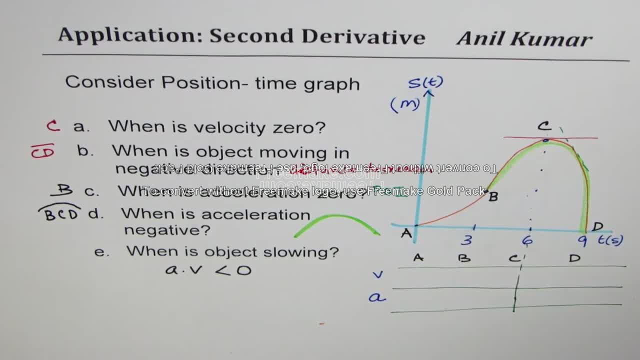 and acceleration a. so from a to c, velocity is positive in this portion, but from c to d it's is negative. This is about velocity. As far as the acceleration is concerned, it is concave up in this portion right A to B. it is concave up. That means acceleration is positive right. 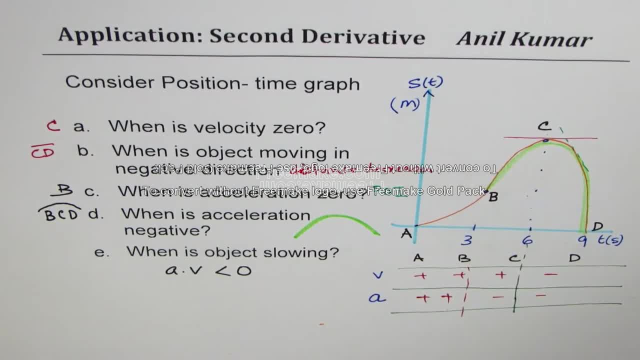 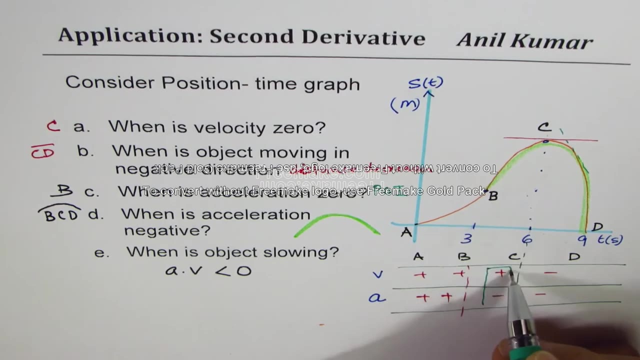 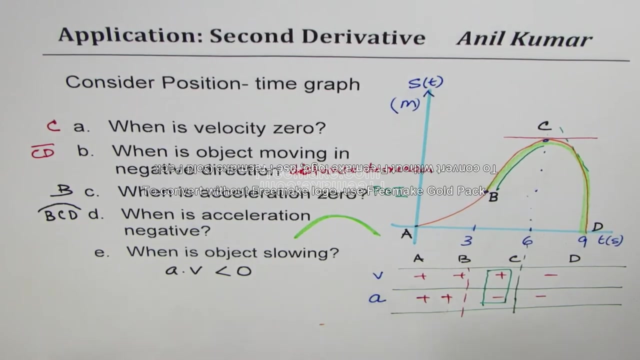 From B to D, it is negative. Now when we say when is the object slowing down, in that case they should have opposite signs. So the only opposite sign combination which you get is in this portion, B to C. right, So B to C is the portion when the object slows. 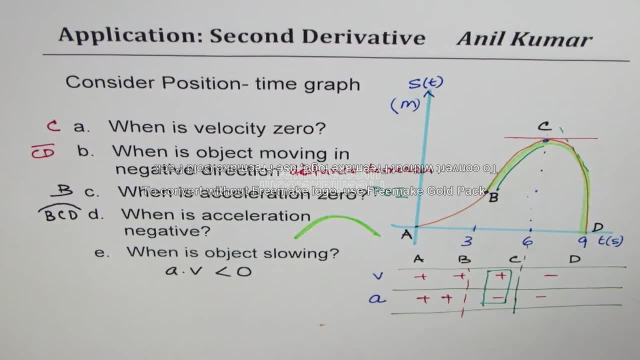 down. Is that clear to you, right? So the answer here is from B to C. The object slows down, So you have to analyze both velocity and acceleration. answer such a question, right? so I hope you find it interesting. let's move on to. 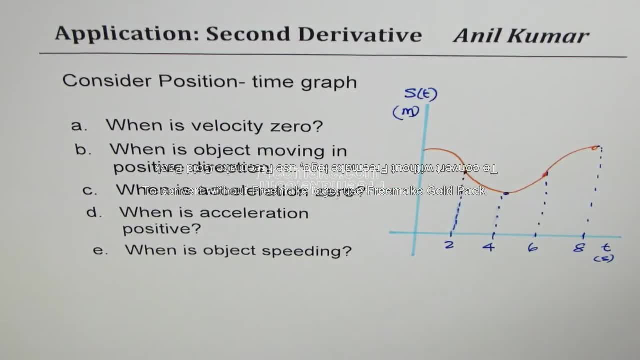 the next graph now. okay, so here we have another curve, which is also a position time graph. you need to answer the same five questions: when is velocity 0, when is object moving in positive direction, when is acceleration 0, when is acceleration positive and when the object is speeding, this time speeding. 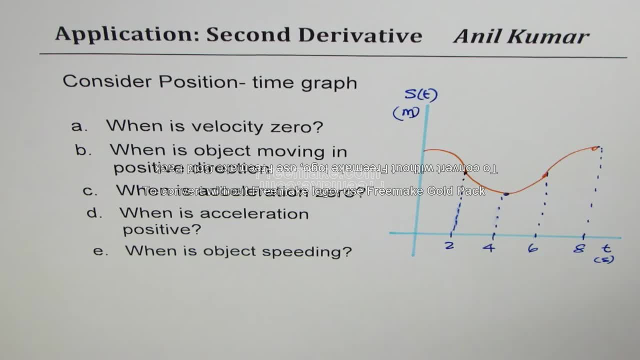 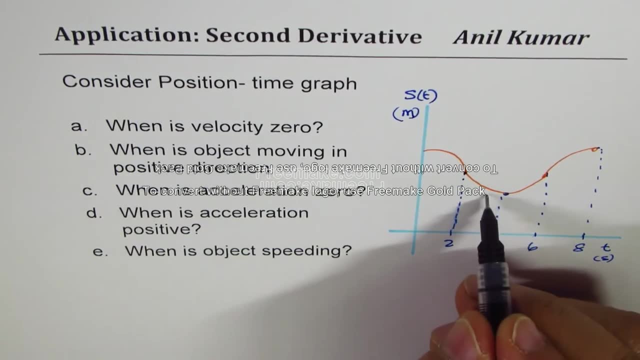 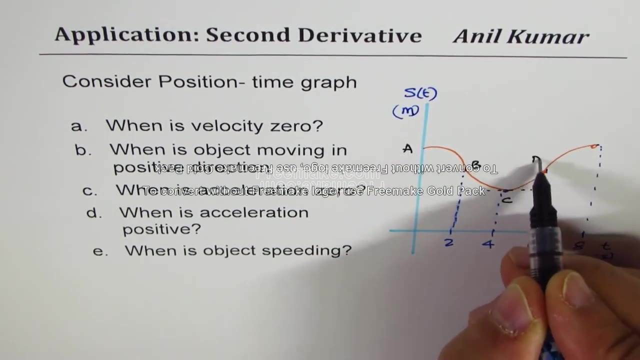 okay, so you can pause the video, answer the question and then look into my sedations. so for zero velocity, we are looking for tangents to be horizontal. so it is okay, this first number. so a, B, C, D and E are our points. so velocity is 0 at. 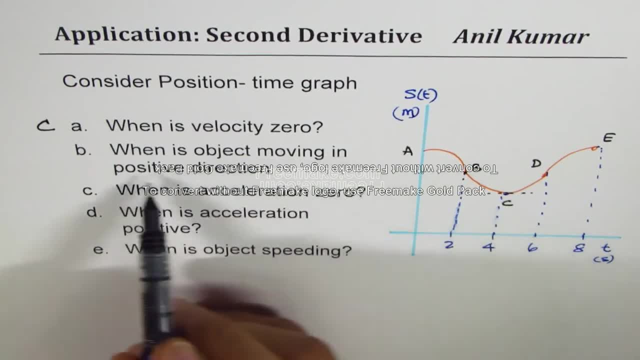 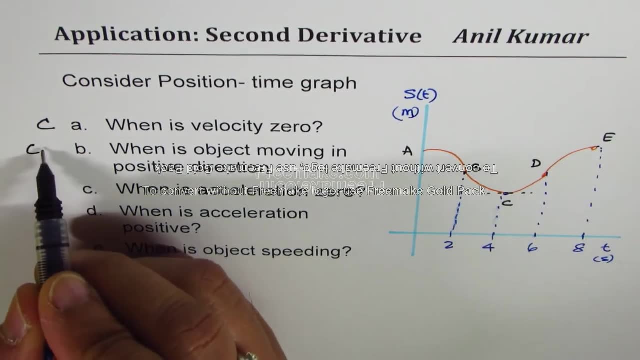 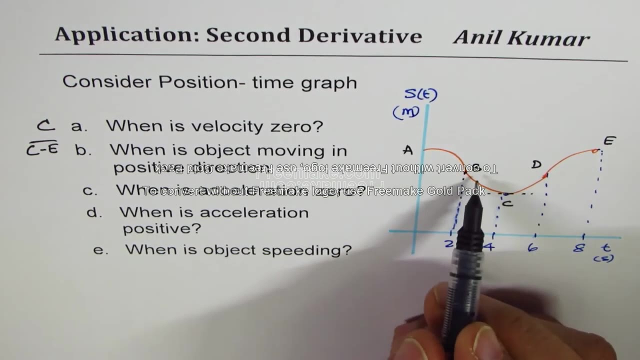 you can see clearly: C, when is object moving in positive direction means going away, right, so it is from C to E. right so it is from C to E. right, so it is from C to E. it is wrong, see to ease it. okay now, when is acceleration 0? we are looking for point of inflections, which is B and D, right so? 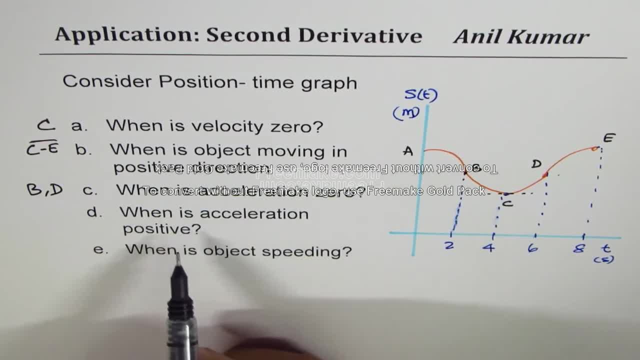 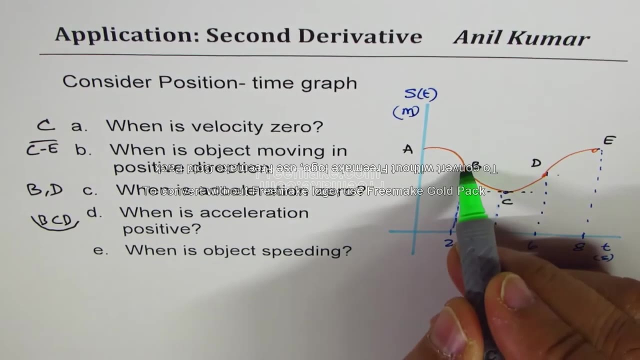 it is B and D when his acceleration positive. positive means concave up, so it is B C D. so it is B C D, is it okay? so that is concave hour. let me draw like this: so This is concave up where acceleration is positive. right. 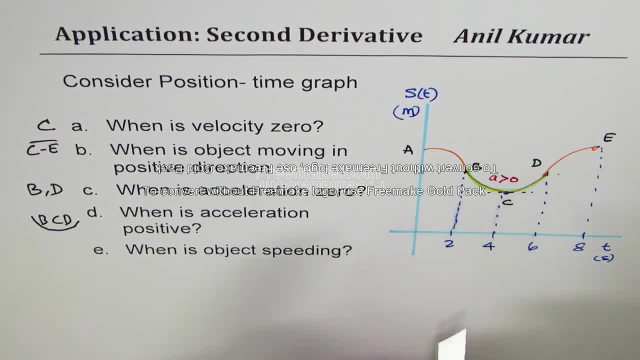 So a is greater than 0.. In other portions a is negative. Now it says: when is object speeding? That's interesting part which we'll discuss now. For speeding, both acceleration and velocity product should be same, And when you multiply you get something which is greater than 0. 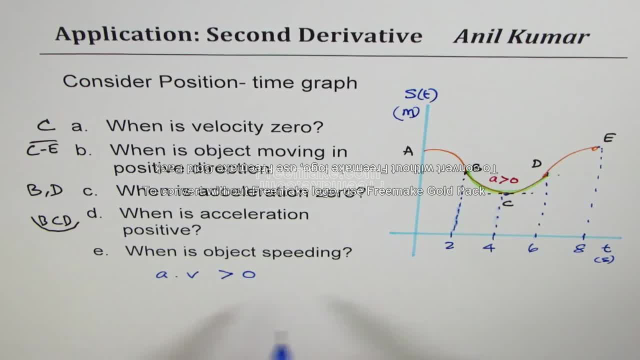 So that is the strategy, okay. Now in this diagram you have to figure out where the velocity is positive, where is acceleration is positive and where are the negative. So let me write down Here: the acceleration is negative. 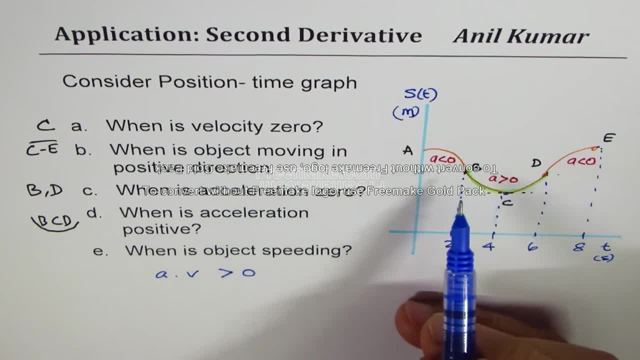 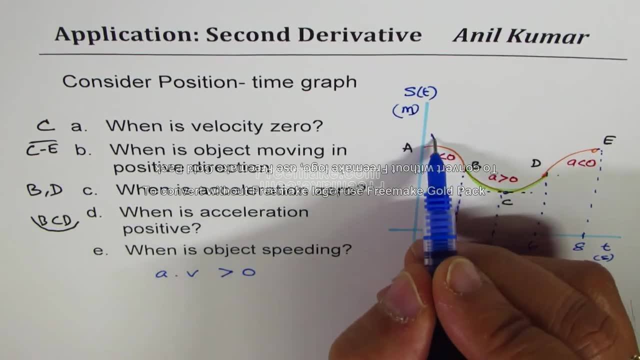 Here acceleration is negative And use another ring to write velocity. So, as you see from this portion, since if I draw a tangent line, velocity is less than 0,. velocity is less than 0. It is 0 here. 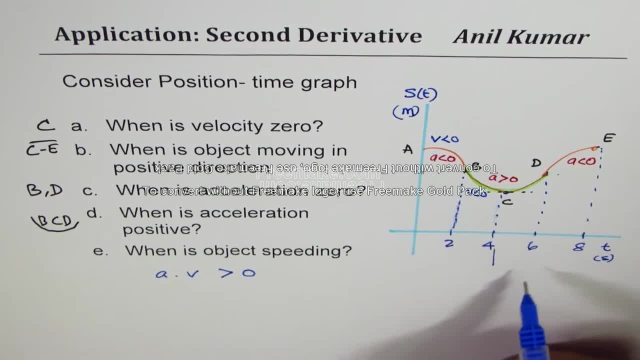 But then it is positive, So in this portion. so what we have here is let me extend here kind of let me extend here and then do So in this portion. velocity is greater than 0, right.